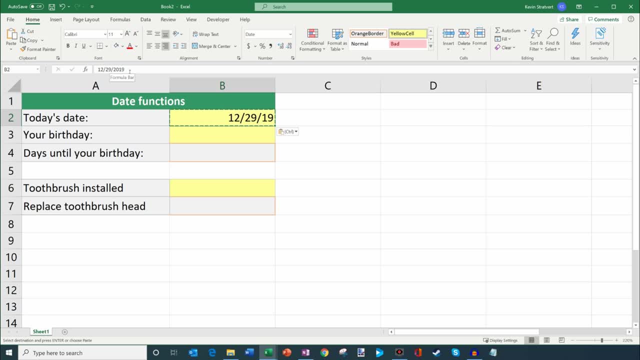 value. you'll see that the formula has gone away and now it just keeps that date static. So that's one day that I could keep it. I just undid that, So it'll show today again. Now what I'm gonna do next is I'm going to enter in my birthday- My birthday is August 11th- And then I'm going to go. 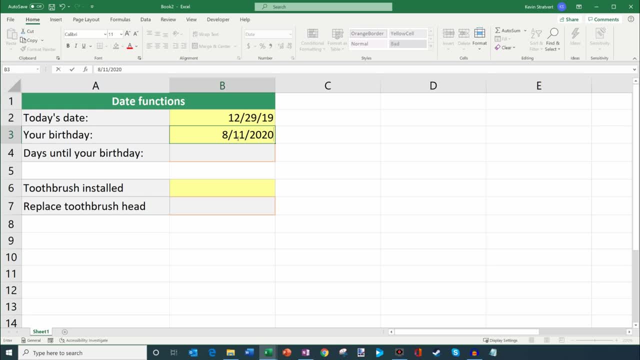 to August 11 and it's coming up on August 11, 2020.. And that's the next time my birthday takes place And I'm going to hit enter. So how many days are in between August 11 and then today? 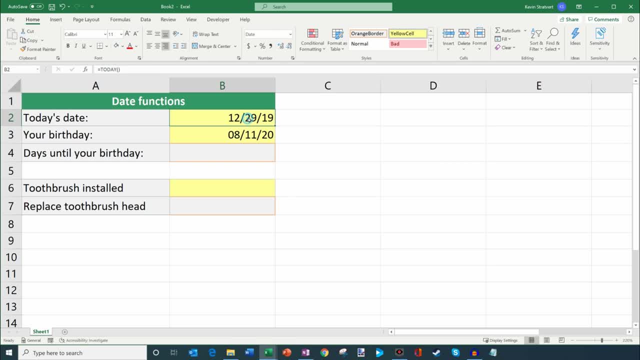 1229.. Well, what we could do is the great thing is you could simply take one date and subtract another date from it. So what we're going to do is we're going to enter a formula, And to do that, I'm going to type in the equal sign. That's how you always enter a formula in Excel And then 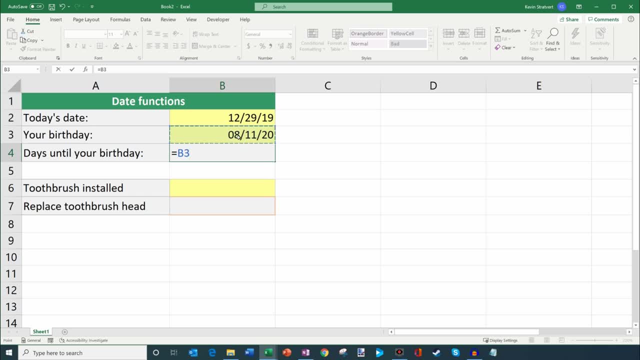 what we're going to do is we're going to select cell B three. That's my birthday, So my birthday is on today. So we want to take the bigger number and subtract the smaller number. So now what we're going to do is I'm going to subtract today's date from my birthday, So B three minus B two. 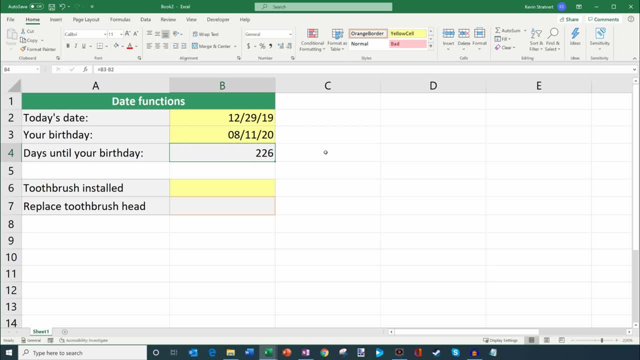 and then I'm going to click on enter And it tells me that there are 226 days left until my next birthday. So I'm I get to be this age for a little while longer before I get older again. Now, one of the things that's interesting. So here you'll see these dates in Excel. 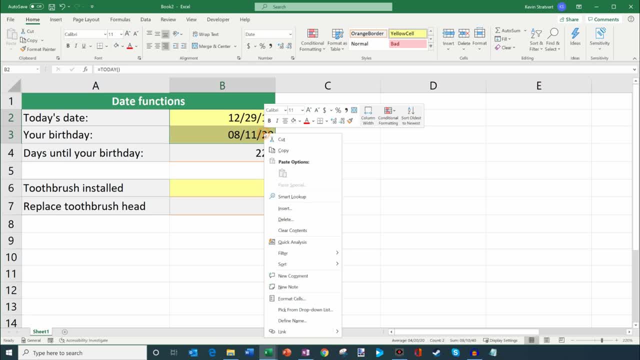 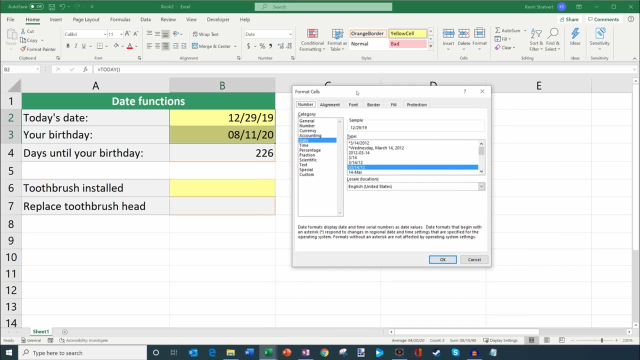 uh, the way Excel calculates the numbers in between these. So here, if I click on, I just hit my right mouse button And what I could do is I could go to format cells. right now It's set to the date format, but I could also just go to number format and I'm going to do no decimal. 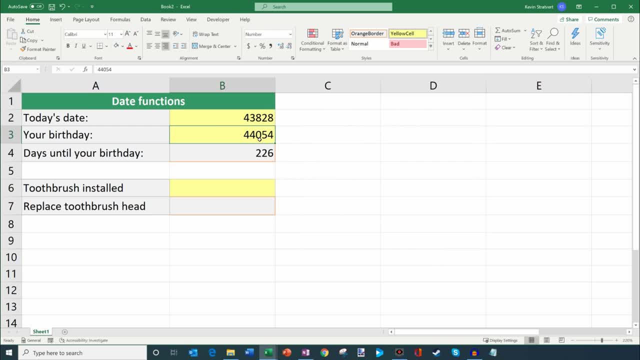 places and then click on Okay. So Excel. what it does is it takes eight, 11, 2020, and it takes today's date of 12, 29,, uh, 2019.. And it converts these into a number, And so here you'll see that. 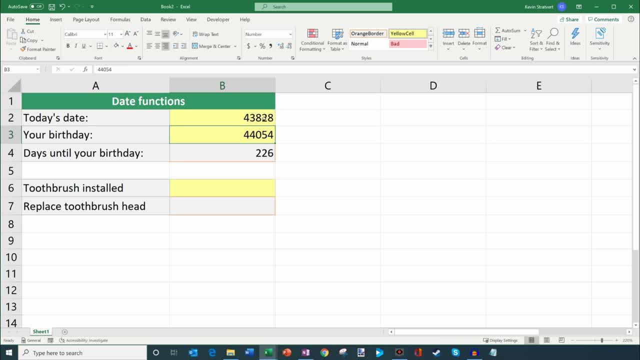 my birthday is on basically day 44,054, and then it subtracts today's date, which is 43,828, to get 226.. Now, interesting fact about Excel: Excel starts its dates on January 1st 1900.. So if I 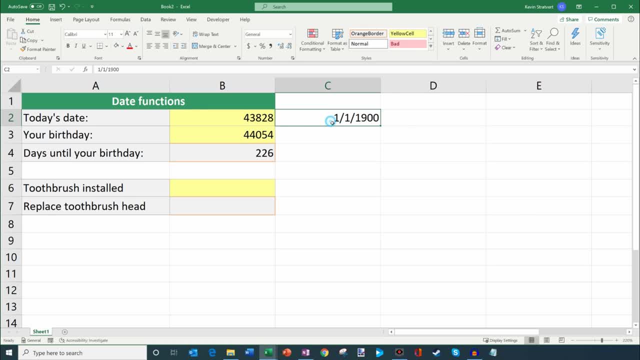 type in one one, 1900,. uh, so I've entered a date, but if I now format that to a number, you'll see that this is day one. Um, so day one is in the early 1900s, or is 1900.. I'm gonna go. 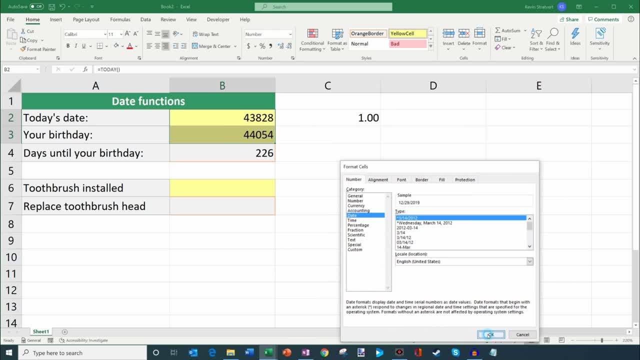 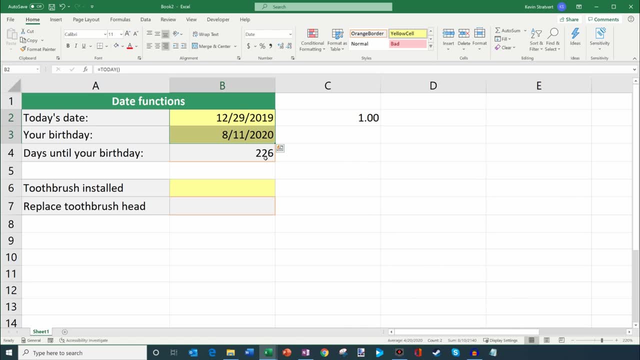 ahead and let's format these back to a date. So I'm gonna go ahead and format these as a date again And there we go, So the date shows up. Now what you can also do is- this example is subtracting dates from one another. What I can also do is I can add dates. So here: 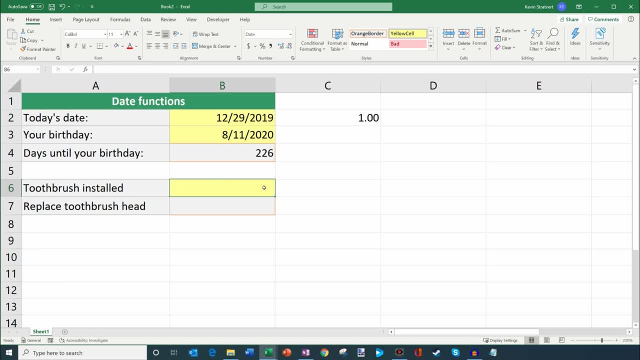 uh, you know, I have a Sonicare toothbrush at home and they always recommend using it for about I think it's about maybe three months or so before replacing your toothbrush head, But when that is, this is always a mystery to me. I always just keep going until it looks like it's gotten a. 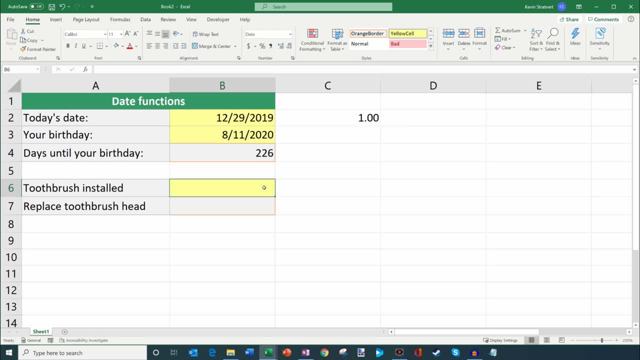 little older, Uh, but today maybe I could use a spreadsheet to really help me stay on top of that. So what I'll do is, let's say, I installed a new toothbrush head today. So 12,, 29,, uh, 12, uh. 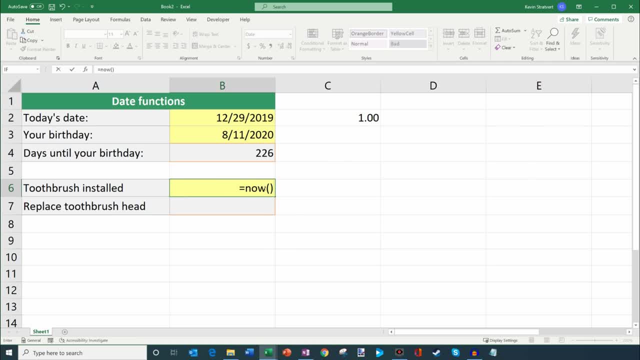 I'm gonna go ahead and enter that in. What I could also do is I can type in: now that's another formula you know, and that'll give me today's uh date and time. So I entered that in. So 12,. 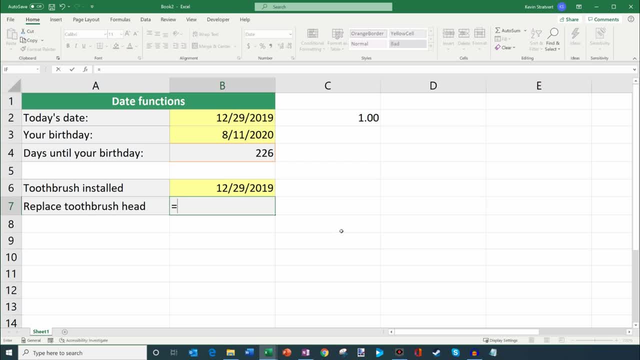 29, 2019.. And what I can do then is I'm gonna type in a formula So we'll do equals today's date And let's see. I think they always recommend about three months, So that's about 90 days. 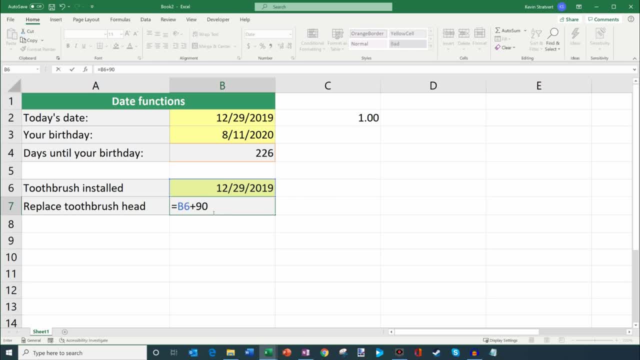 So I'm gonna add 90 to it. So I'm taking this date and then adding 90 days, And so now what it tells me is that's end of March. So three, 28,. 2020 is in about 90 days. 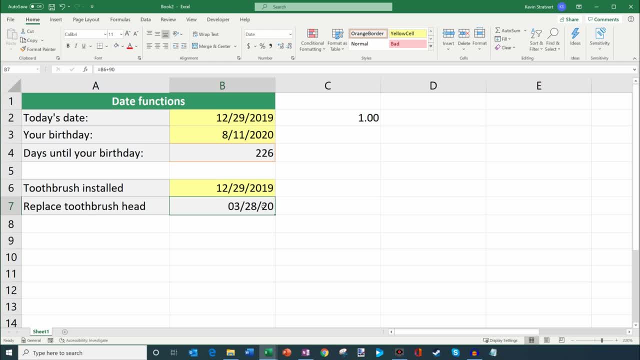 So this will remind me. okay, so I need to replace my toothbrush head on this date. Now I I showed two different formulas as we were going through this. One of them is: today I'm gonna go ahead and type that in, So type in that formula, And then I'm also gonna type in: 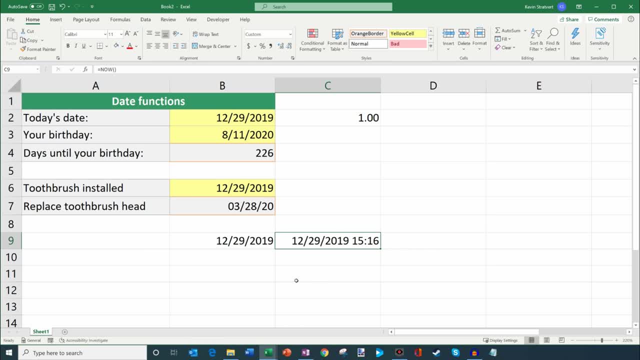 this other one I typed in, which is now, what's the difference? Well, the difference is: today will show you just the date. today, Now, will not only show me the date, but it'll also show me the time, So it gives me a little extra detail. um, when I type in either one of those formulas, 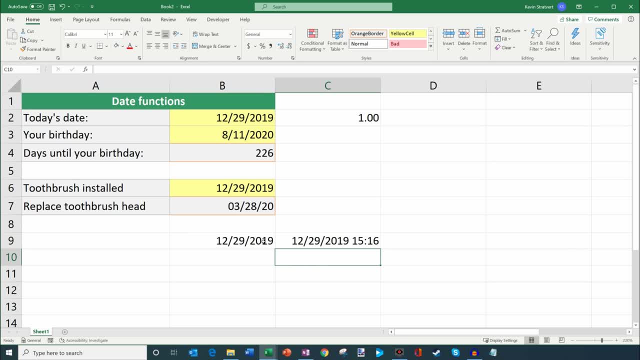 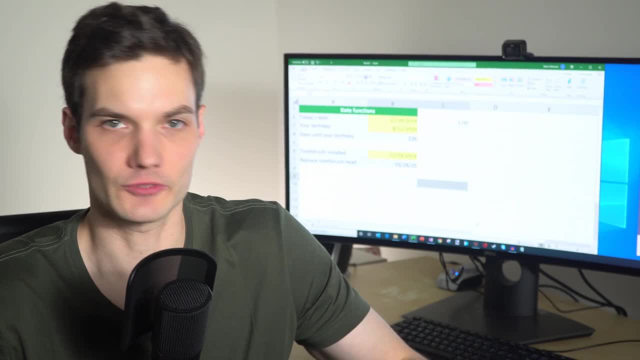 but those are two different ways, uh, to get the current date and or time to show, All right. Well, that's how you work with dates in Microsoft Excel. You could very easily add dates, You can subtract dates, Uh, and hopefully. 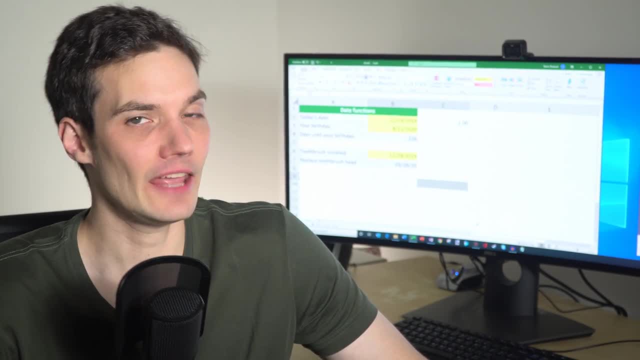 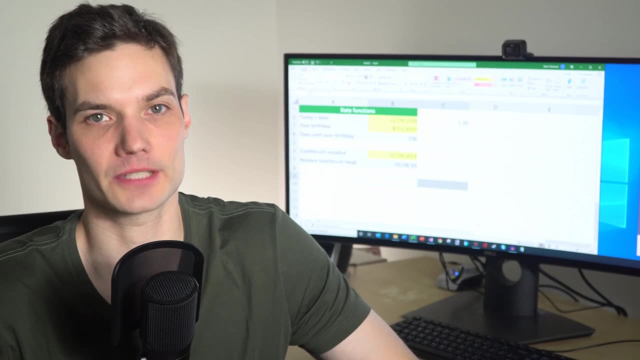 you're an expert working with dates in Microsoft Excel. Now, if you feel like you are an expert working with dates, please give this video a thumbs up. If you wanna see more videos like this in the future, please hit that subscribe button. That way you'll get a notification. 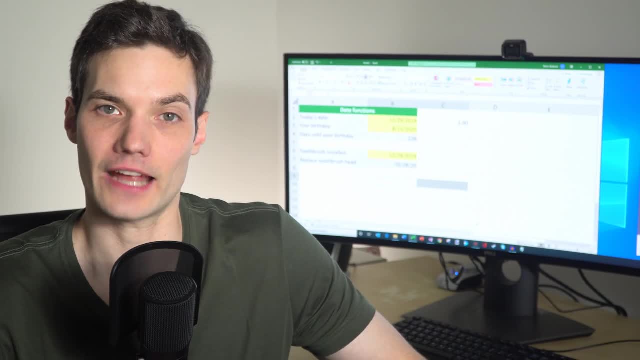 Anytime new content like this comes out. And lastly, if there are any other videos that you wanna see me cover on my channel in the future, leave a comment down below. I take a look at them and I'll add that to my list. 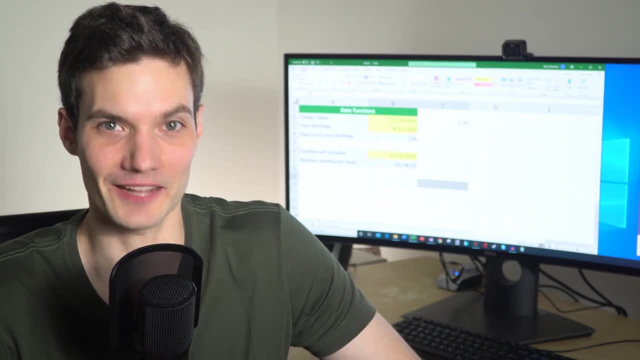 of videos to create, All right. Well, that's all I have for you today. I'll see you next time. Bye. 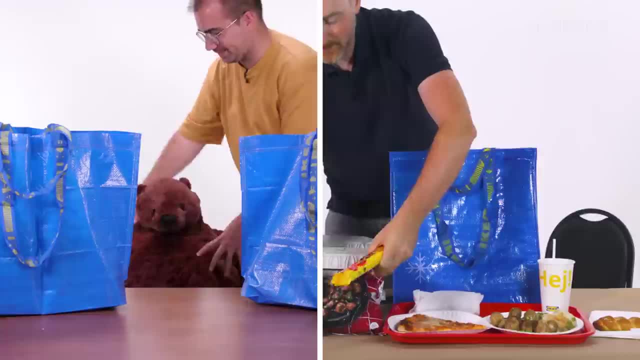 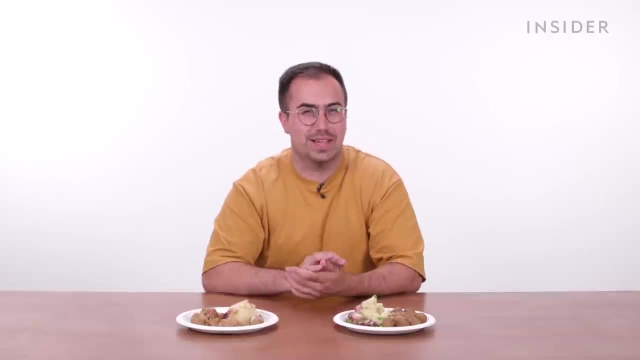 From exclusive items to portion sizes. we wanted to find out all the differences between Ikea food in the US and the UK. This is Food Wars Quick note. it turns out Ikea does not offer a takeout option, but fortunately they do sell lots of Tupperware containers. So in case you're wondering, 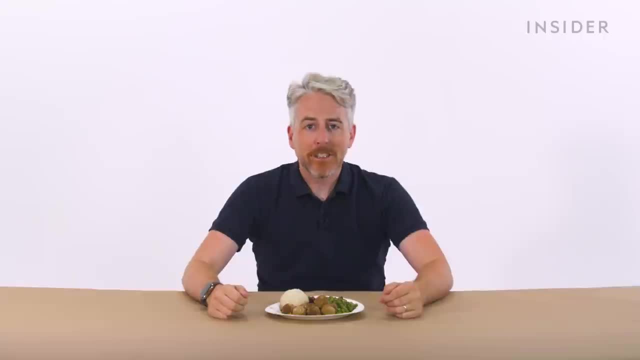 why the food looks a little bit sad, it's because we had to improvise On with the video. Let's start portion sizes with Ikea's claim to fame when it comes to food. the Swedish meatballs In the US Ikea's restaurant offer only one portion size for meatballs: eight pieces, But after that. 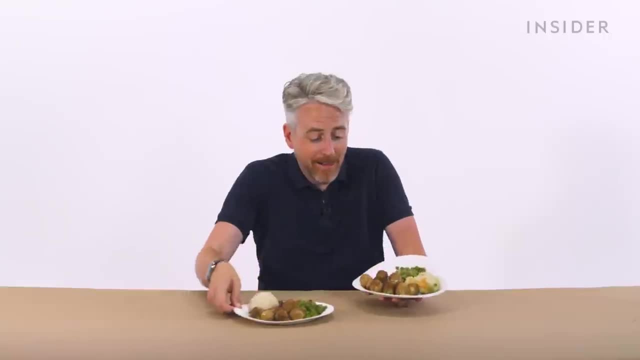 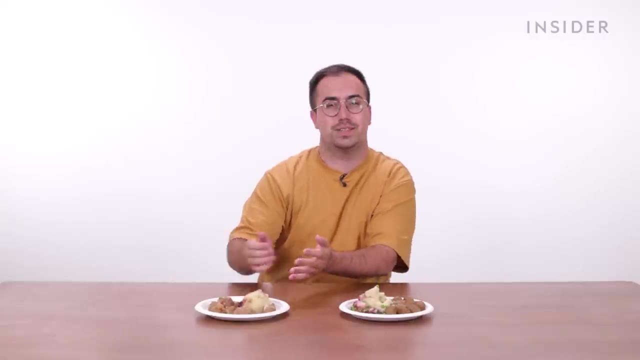 you can get them in increments of four, For instance, 12 meatballs. In the UK, Ikea's iconic meatballs come in two portion sizes: eight or 12.. You can also add four extra meatballs to any order for an extra £1.75, and there's seemingly no limit to how many times you can do this In the UK. 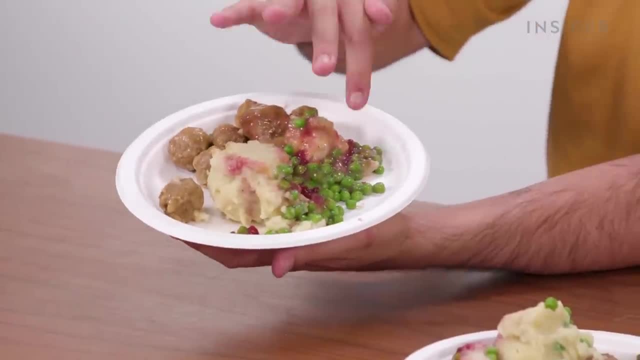 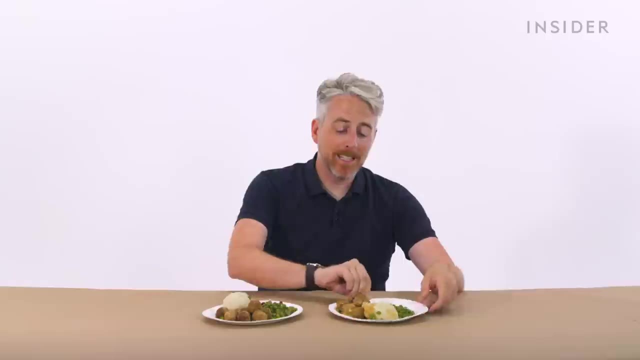 the meatballs come with either mashed potatoes or chips on the side, as well as some garden peas, lingonberry jam and some other ingredients. So if you're looking for something, that's a little and of course, their famous gravy And of course, the meatball options- all come with a side of mashed. 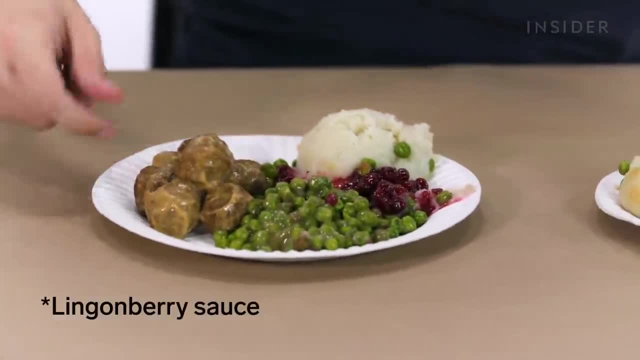 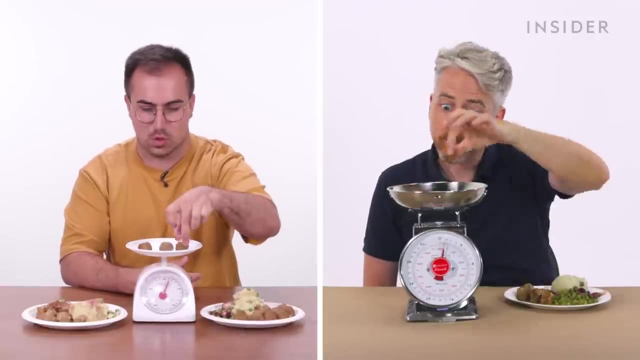 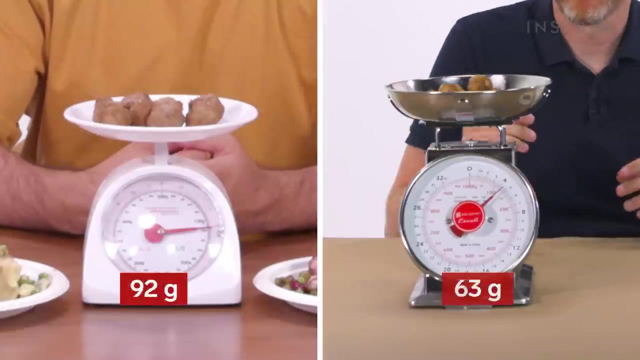